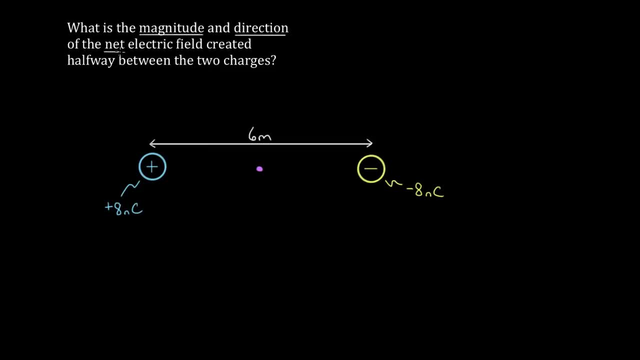 what's the magnitude and direction of the net electric field, ie the total electric field created halfway between these two charges down here. So you've got a positive eight nanocoulomb charge and a negative eight nanocoulomb charge, and they're separated by six meters from the 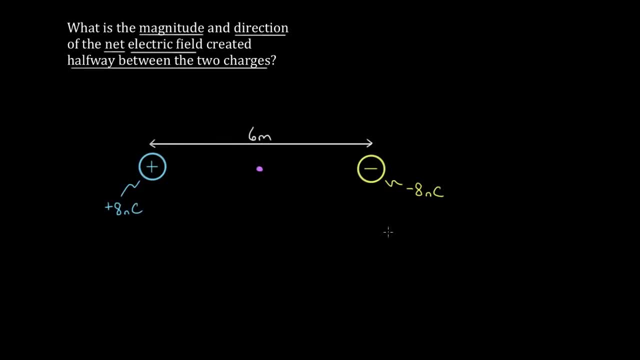 center to center distance. But what we want to know is what's the total electric field that they both create right there? So each charge is going to create an electric field at this point and if you add up, like vectors, those electric fields, what total electric field would you get Now at? 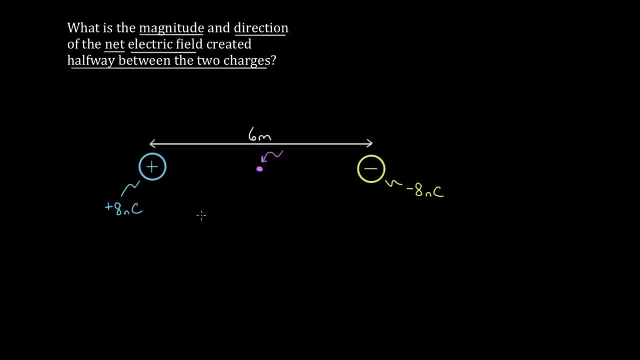 first you might think: well, you should just get zero, right. It's very tempting to say that the electric field is just going to be zero there, because you've got a positive eight nanocoulomb charge and a negative eight nanocoulomb charge. But what we want to know is: what's the total? 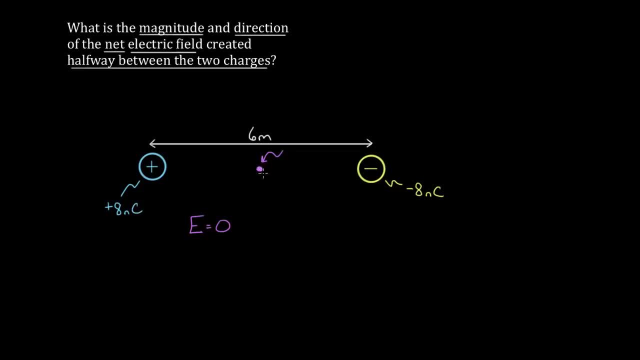 negative eight nanocoulomb charge and those should just cancel, right. But you have to be really careful. That turns out that's not true here. This is not going to be true, And to see why, first you should just draw what is the direction of each field at that point. So this: 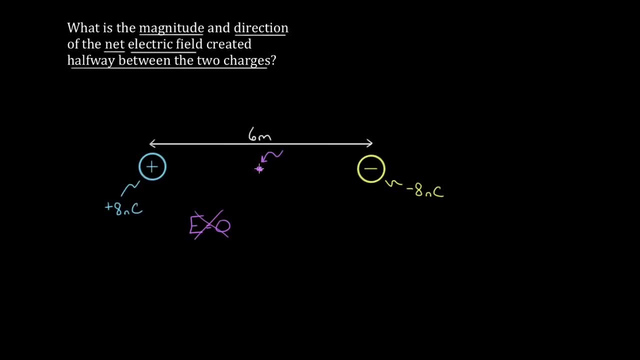 positive eight nanocoulomb charge is going to create a field at this point that goes radially away from the positive charge, and so it's going to go to the right. And I'm not even looking, So when I'm trying to find the electric field from this positive charge over here, I'm not even 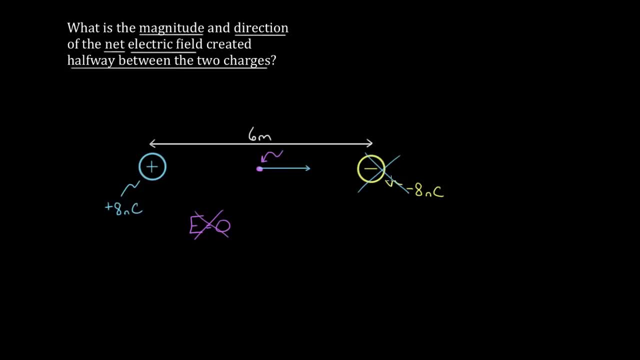 paying attention to this negative charge. I pretend like this negative charge doesn't even exist And I just ask: what field would this positive charge create? It's still going to create that field, whether this negative charge is over here or not, And I can do the same thing. I can ask: 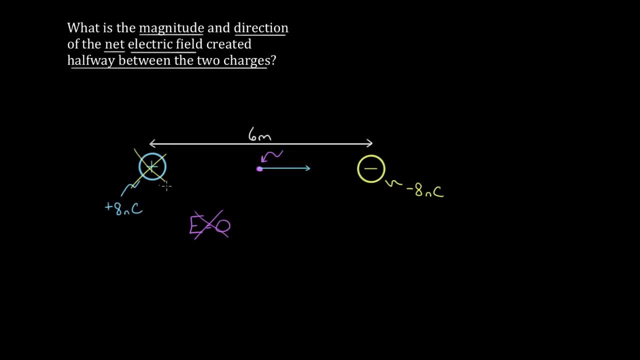 what field would this negative charge create? And I'm going to pretend like this positive charge isn't even here. So negative charges create a field to go radially in. So over here, radially in would point to the right. So these don't cancel The negative charge. created a field radially in. 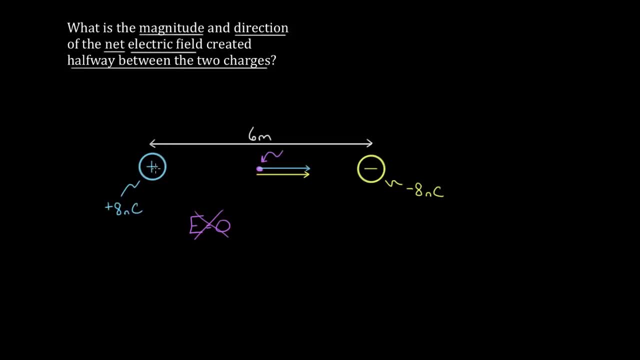 That was to the right. The positive charge created a field radially out of the positive charge. That was to the right. So not only are these not going to cancel, these are going to add up to twice the field. because you're going to add up these vectors, You just add them up if they're in the same. 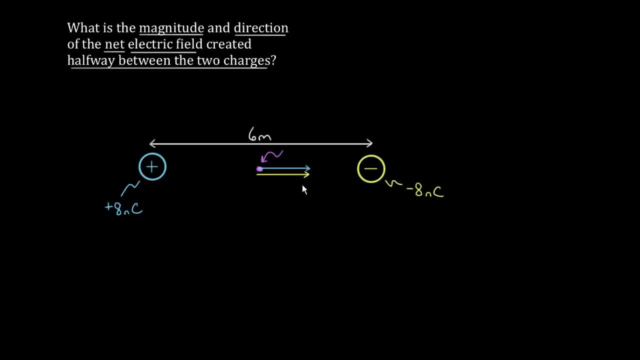 direction and you get two times the contribution from one of them. So it's not always the case. In other words, it's not always the case that a negative charge and a positive charge have to cancel their electric fields. Those electric fields might point the same direction. so you've got to. 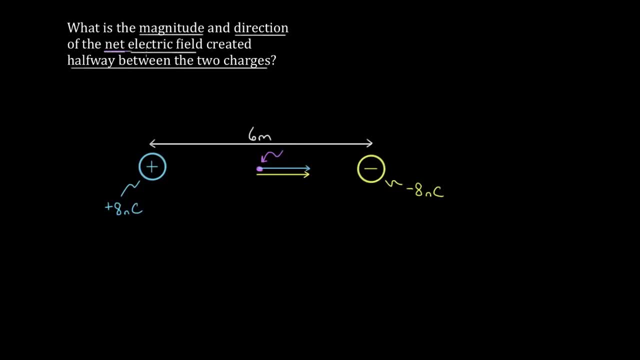 be careful. So how do we find this net electric field then? What do we do? Well, we're going to say that, all right, this electric field. the first thing I could say is: this net electric field is just going to point in the x direction. So this is just really in the x direction, All I. 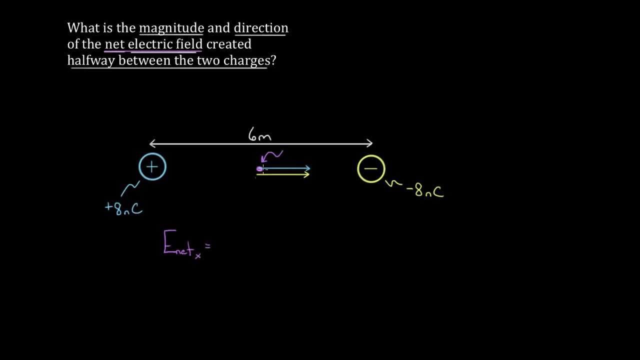 really care about is the electric field in this horizontal direction, and it's going to be equal to the sum of the electric fields each charge creates there. So we'll do the blue charge first. That's going to be k times the blue charge divided by r squared. Then we'll do the yellow. 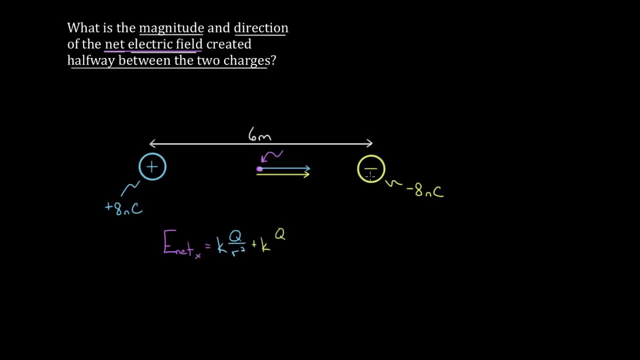 charge. It's going to be plus k, the charge of that yellow charge divided by r squared. So we'll plug in some values here. This k is always 9 times 10 to the 9th and the q of this blue charge was: 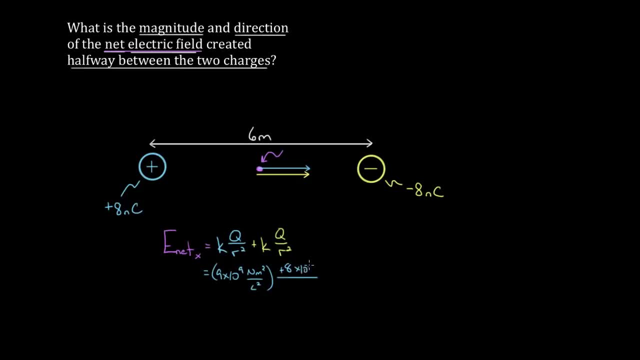 positive 8: nanocoulombs. Nano is 10. to the negative 9th. I like using nano because then that negative 9 cancels with that positive 9.. And what distance do I put in here? A lot of people want to. 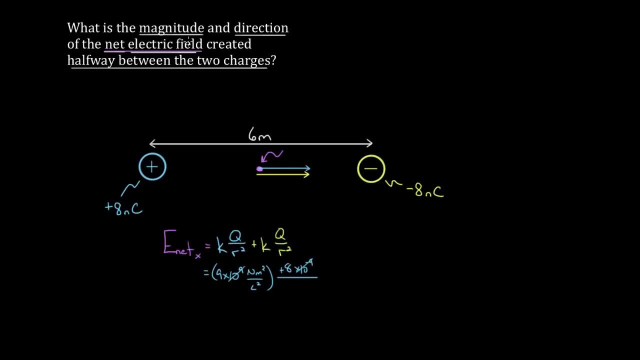 put in 6, but that's not what I want. Think about it. I want the net electric field halfway between the two charges. So the r that I care about in this electric field formula is the distance from the charge to the point where I want to determine the electric field, And in that case this is 3. 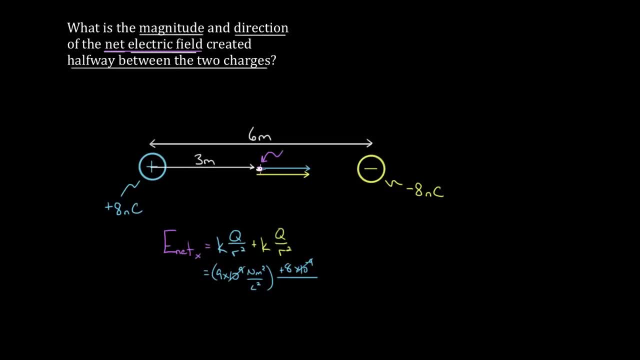 meters. So for this case, from the charge to the point I'm concerned about, I'm finding the field is 3 meters, not 6 meters. If we were finding the force these charges exert on each other, then I'd have to use 6 meters. But that's not what I'm finding. I'm finding the field. 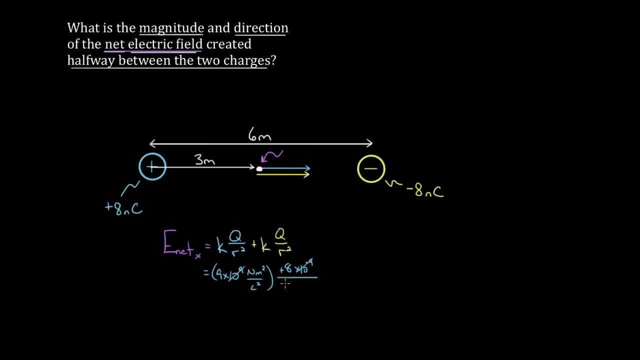 each charge creates at this halfway point. So I'm going to plug in 3 meters down here and I can't forget to square it. And now I have to be careful. Just because my charge is positive doesn't necessarily mean that the contribution to the electric field is positive. You have to. 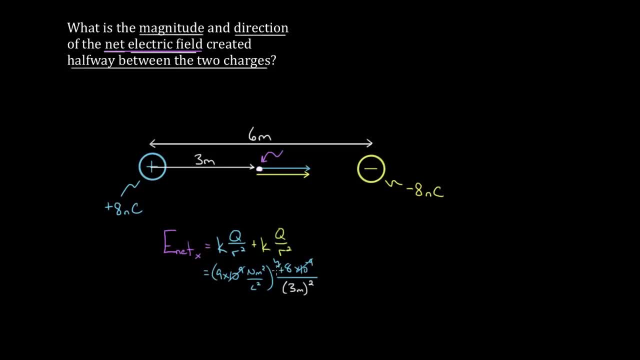 check. You can't rely on the sign of this charge to tell you whether the contribution is positive or negative. I've got to look at what direction it points. The direction this positive charge creates a field is to the right, Since that's typically 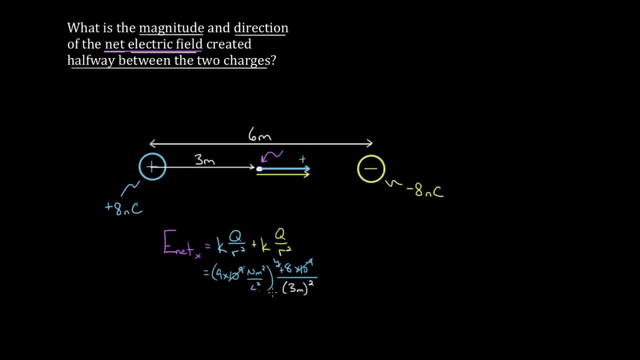 the direction we call positive, then I'm okay with calling this entire term here positive, And then we're going to have another term. I'm going to leave off the plus or minus, because I mean it might be plus, it might be minus. We'll leave that off for a second. We'll have 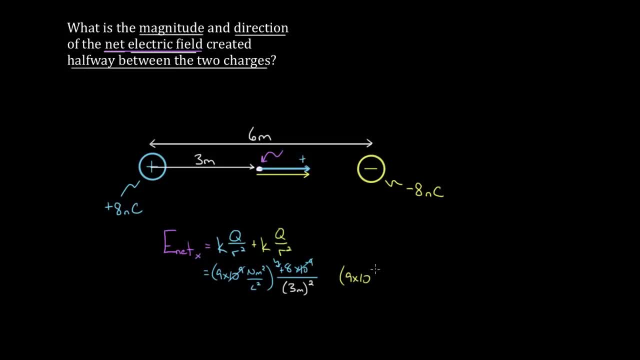 to decide when we know what direction it goes. So we do 9 times 10 to the 9th And then the charge is negative 8 nanocoulombs. but I am not going to plug in the negative sign, Oops. 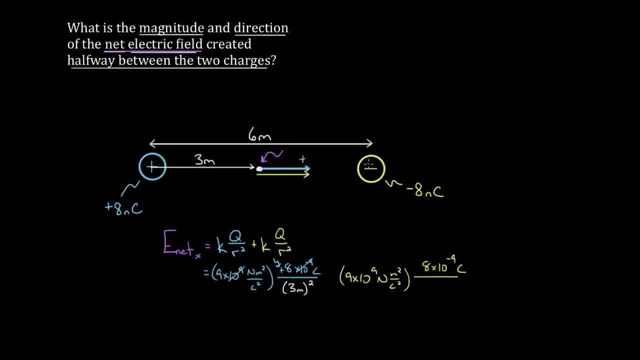 and I left off coulomb on the other one here, Sorry. And then again, the distance I want is from the charge to the point where we want to find the field. So I'm going to plug in the field And that again is 3 meters, And we can't forget to square it. So should this contribution 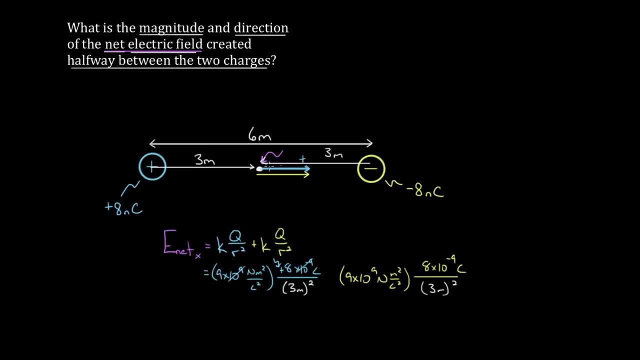 be positive or negative. I can't rely on the negative sign to tell me that I've got to look at what direction it goes, Since it goes to the right. that's the positive direction. So this is going to be plus. These add up. These both go the same direction: the positive direction. So the 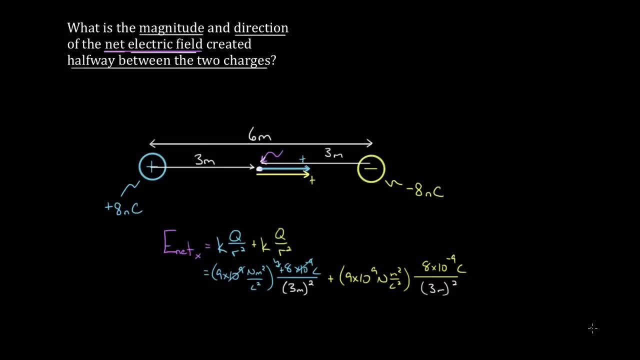 total net electric field is just going to be both of these added up. So if I do this, if I square this 3, I'd get 9. And 9 divided by 9 is just 1.. So I get 8 newtons per coulomb. And then this term. 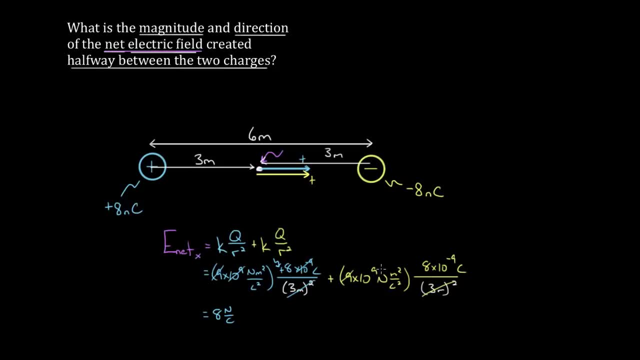 is really the negative sign. So I'm going to plug in the negative sign. So I'm going to plug in the same thing. 9 is divided by 9.. So that goes away. 10 to the ninth cancels with 10 to the. 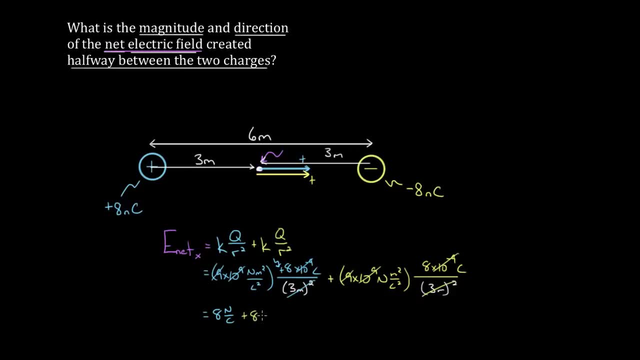 negative ninth, And all I'm left with is this 8. So it'd be plus 8 newtons per coulomb. So each charge is contributing 8 newtons per coulomb of electric field at this point, which means that 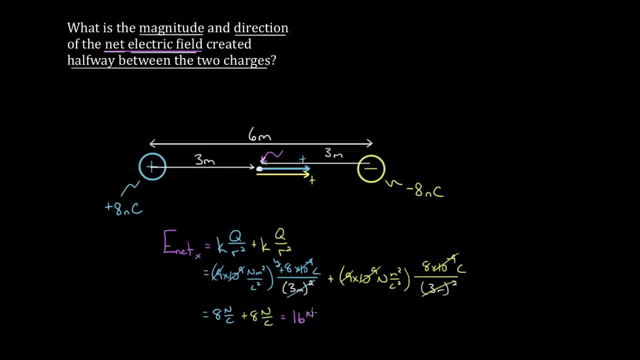 the total net electric field would just be 16 newtons per coulomb at that point. That is the net electric field. That's the magnitude of the net electric field at that point. between them, And which way does it go? What's the direction? It goes to the right. 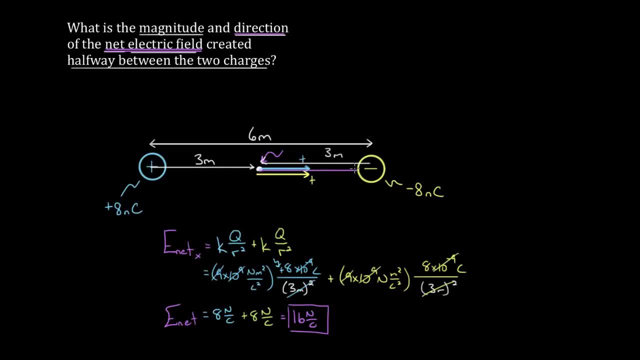 these vectors pointed to the right, So the total is going to be twice as big as one of them, and also to the right. Now if you have a case like this and both terms- you know both terms are going to be equal- You can just write one of them down and multiply by 2. You don't have to just add. 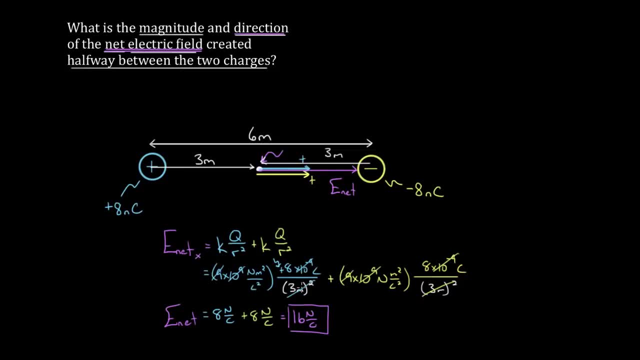 them both up, But I wanted to show you this way so you can see how everything works out. And in the end we get 16 newtons per coulomb for the total field which points to the right. Now what if we changed this? What if we made this instead of a negative 8 nanocoulomb charge? 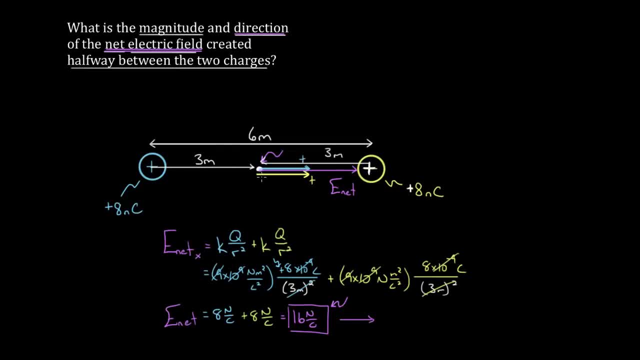 we made this a positive 8 nanocoulomb charge. Well, no longer create an electric field that points to the right Positive charges. create fields that point radially away from them. So it would create its electric field to the left, which means down. 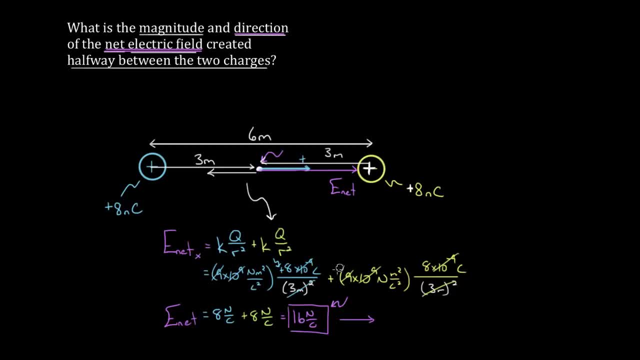 here. when we find its contribution to the electric field, we'd have to include it as a negative contribution because it's pointing in the negative direction. Even though it's a positive charge, the contribution it gives to the total electric field is negative because it points in the